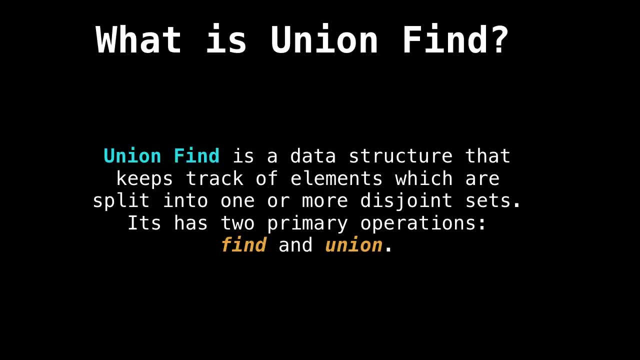 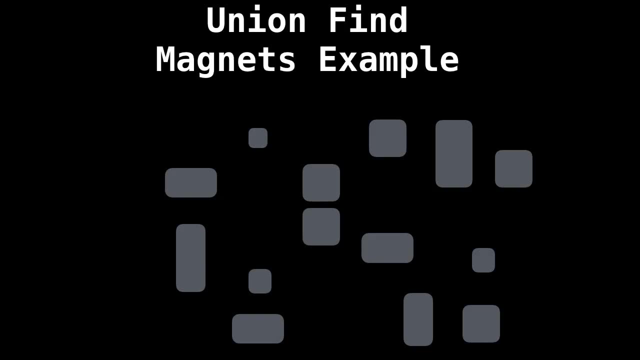 union find will tell you what group that element belongs to. And union merges two groups together. So if we have this example with magnets, suppose all these gray rectangles you see on the screen are magnets, And also suppose that the magnets have a very high attraction to each other. 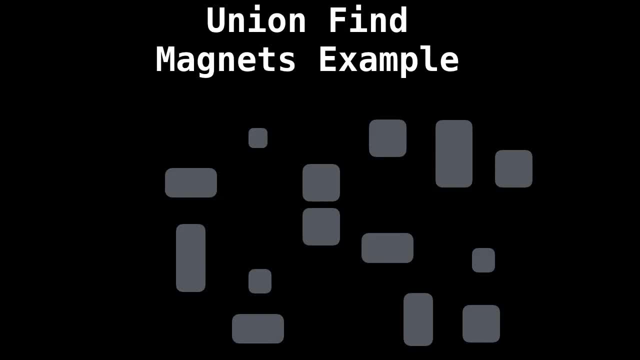 meaning they want to merge together to form some sort of configuration. So if I label all the magnets and give them numbers and we start merging the magnets with the highest attraction first, we're going to merge six and eight together, since they're the closest. 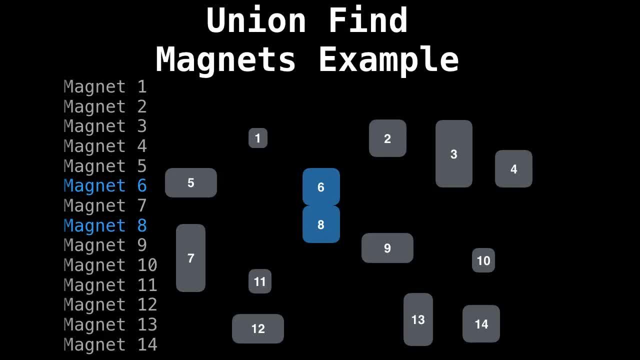 So in our union find- we would say union six and eight, And when we do a lookup on to find out which Sasha groups 6 and 8 belong to, they would belong to the blue group. Now, perhaps 2,, 3, and 4 are highly attracted to each other so they would form a group. 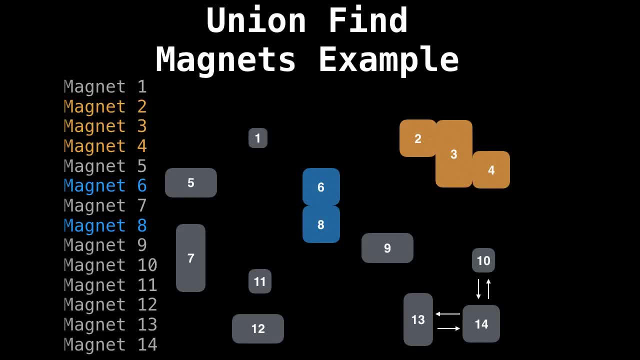 So they would form the yellow group And perhaps 10,, 13, and 14 would also form a group. And this keeps on going and we unify magnets into groups And perhaps we merge some magnets onto already existing groups. So we unify a gray magnet, which is just a magnet in its own group, into an already existing. 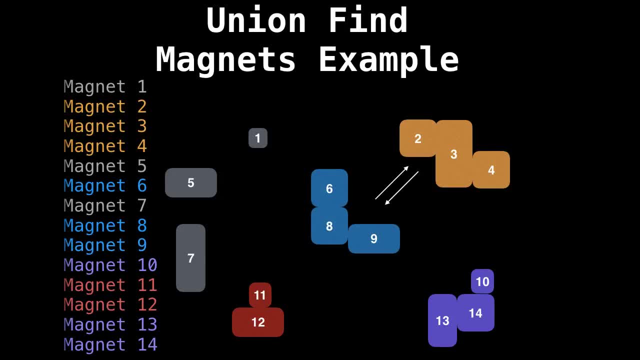 group. But also we can unify groups of magnets which are different colors And then we assign it an arbitrary color, so blue. so suddenly everything in the yellow group went into the blue group. And now when we would do a lookup in our union, find to determine which group say 2,, 3, or 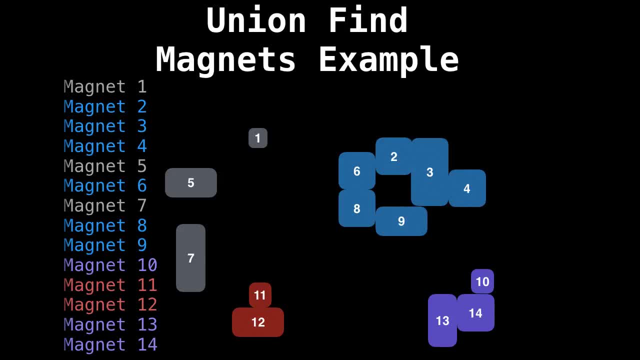 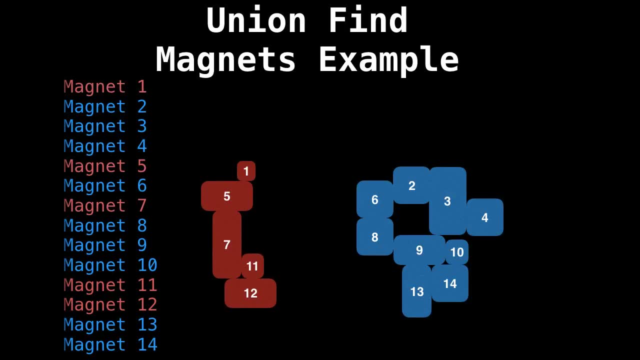 4 are now, we would say, ah, you're in the blue group And the union find does all this merging and finding in a very efficient manner, which is why it's so handy to have around. I'm not explaining currently how that works. we'll get into that in a later video.